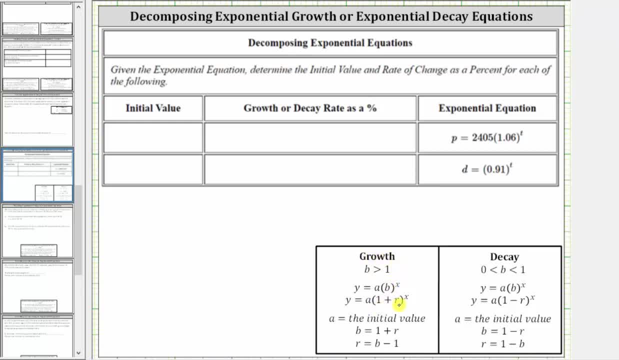 we have exponential growth and the base b is equal to one plus r, where r is the growth rate as a decimal. If we set the base b equal to one plus r and solve for r, we have r equals b minus one And the value of a gives us the initial value. 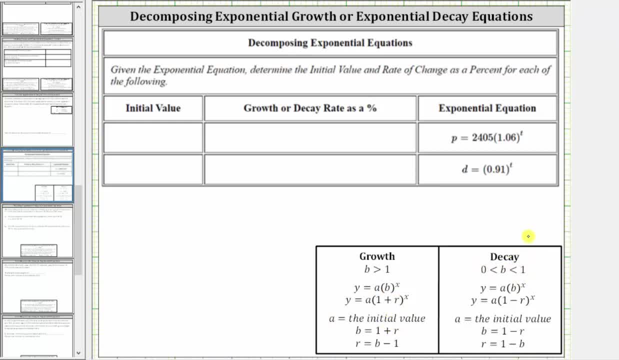 or starting value. If the base b is between zero and one, we have exponential decay and the base b is equal to one minus r, where r is a decay rate as a decimal. And if we set b equal to one minus r and solve for r, 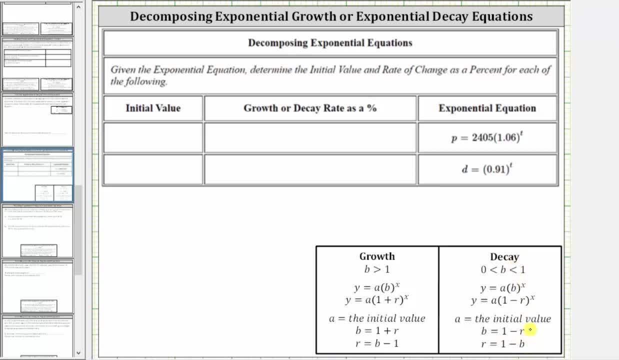 we have r equals one minus b when we have exponential decay, And the value of a is equal to the initial or starting value. So, looking at our first equation, we have p equals 2,400 and 405 times 1.06 raised to the power of t. 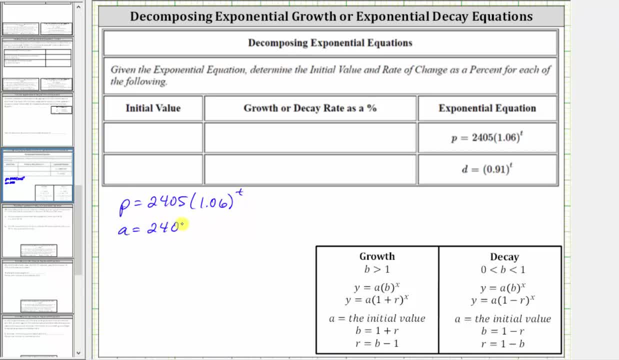 So a the initial value is 2,405.. The base b is equal to 1.06, which is greater than one, and therefore we have exponential growth. And because we have exponential growth, the growth rate as a decimal is r. 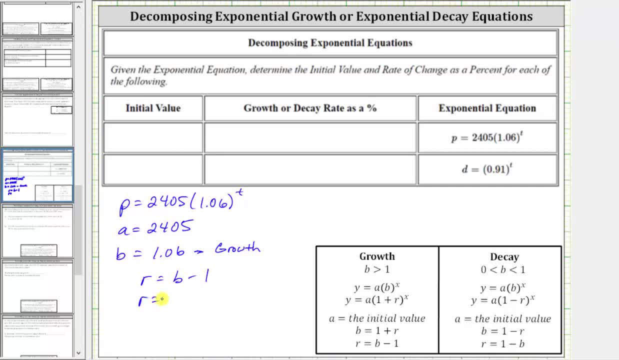 which is equal to b minus one. So we have: r equals 1.06, which is equal to 0.06, which, as a percentage, is 6%. To complete the table, the initial value is 2,405.. We have exponential growth. 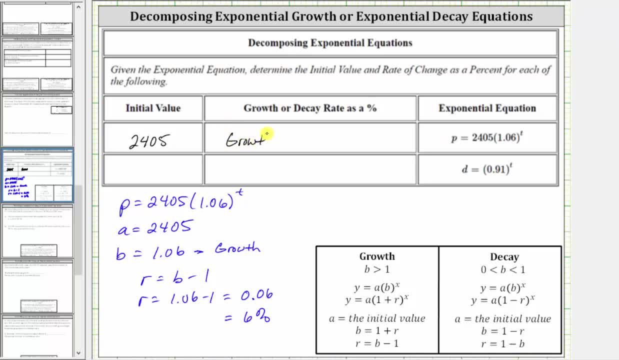 and therefore the growth rate is 6%. The next equation is: d equals 0.91 raised to the power of t. Notice how it doesn't appear as if there is a value for a, but of course we could put a one here, and it's not going to change the values of d. 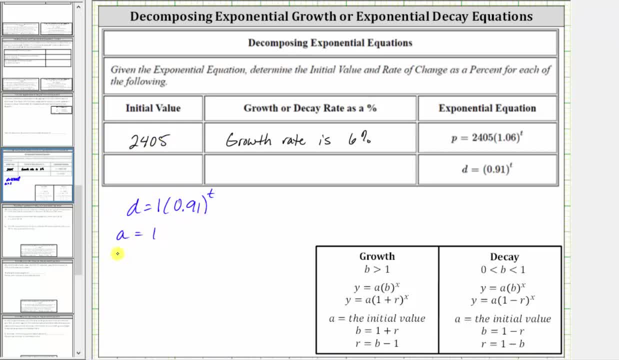 and therefore a, the initial value is equal to one, The base b is equal to 0.91, which is between zero and one, and therefore we have exponential decay this time. And because we have exponential decay, the exponential decay rate, r, as a decimal.